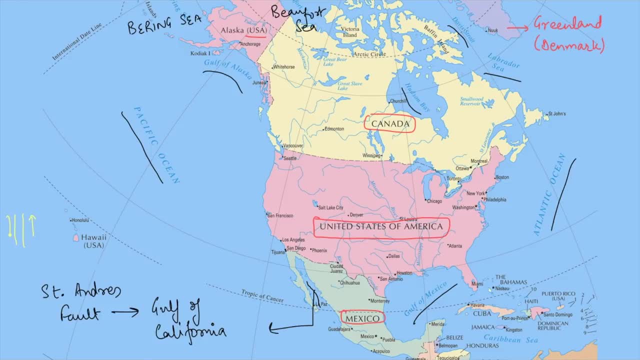 If these two plates move in the opposite direction, then the earthquakes that occur due to their friction are due to transform boundaries. So these are transform boundaries. Generally, tectonic plates converge or diverge- convergent or divergent boundaries, But if they move in opposite direction then they are known as transform. 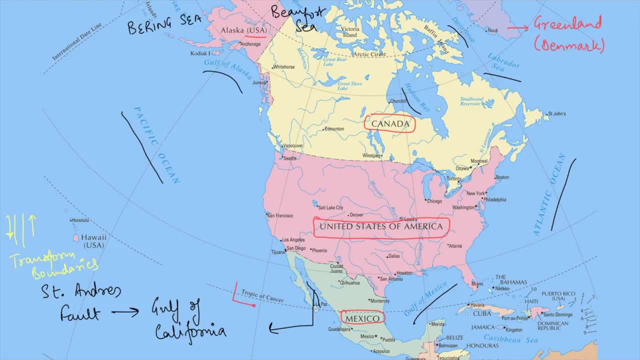 boundaries. Another important thing that we need to know is that the tropic of cancer passes through Mexico and not through USA and Canada in North America, And then the arctic circle passes through USA, Alaska region and Canada and Greenland. Now let us look at the capital cities of these countries. 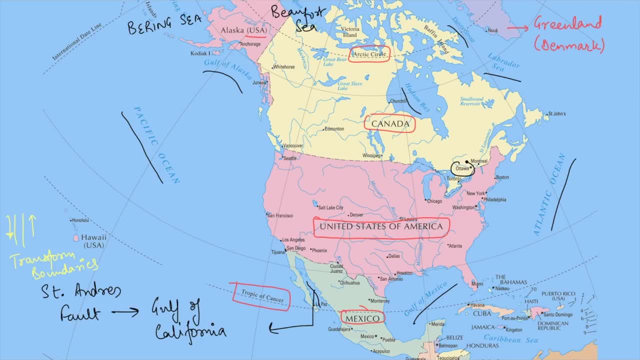 Canada is the capital of Ottawa. Then we have Washington DC in USA, And then we have Mexico and Canada in Japan, And then we have Canada in Canada, Then we have Canada in Canada And then we have Canada in Canada. Washington DC is different from the state of Washington. Washington DC is on the eastern. 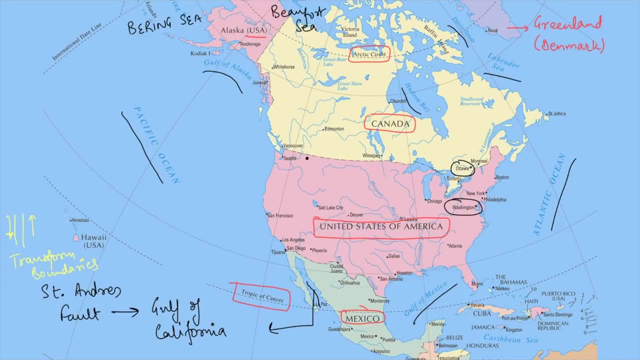 coast of USA and Washington state is on the western coast of USA, capital of which is Seattle. And if we talk about Mexico, its capital is Mexico City. Now comes the boundaries: as you can see, Canada is surrounded by USA, Alaska and the mainland. 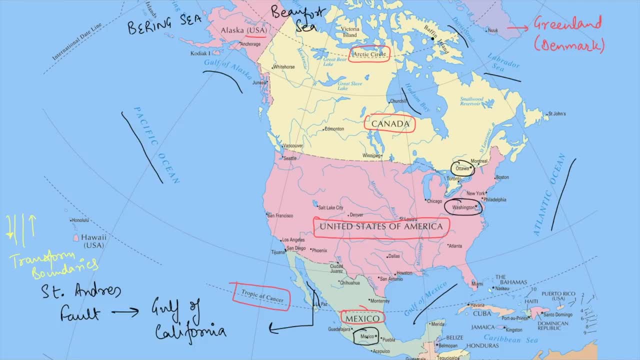 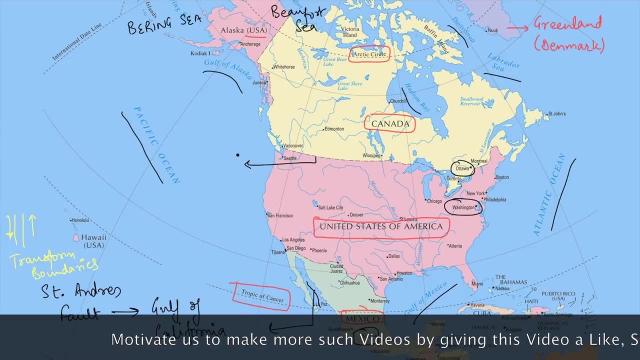 USA, and we can say that Greenland is also a neighbouring part of Canada, whereas USA is surrounded by Canada and Mexico. This boundary, you can see, is known as the 49th parallel Right, so Mexico is surrounded by USA, Guatemala and Belize. 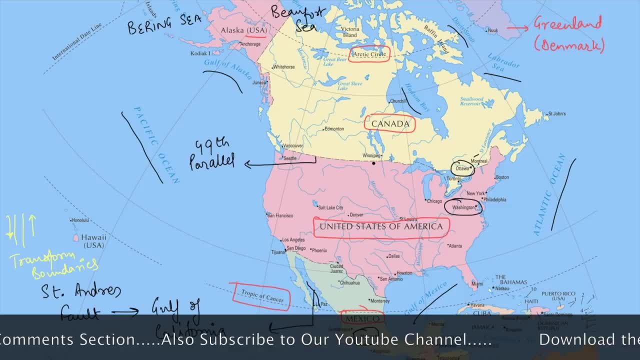 Now let us look at some major cities of these countries. first of all, lets look at Canada. In Canada, you can see Montreal, Ottawa, Toronto, Winnipeg and Vancouver. USA has a lot of cities, since it is a developed country, so there are a lot of developed cities. 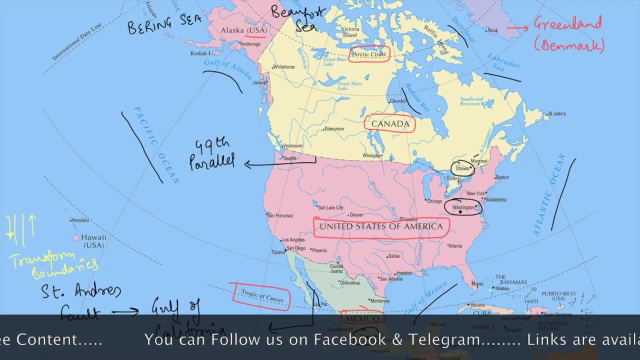 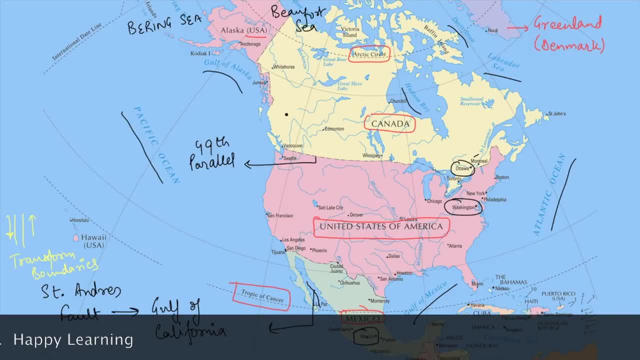 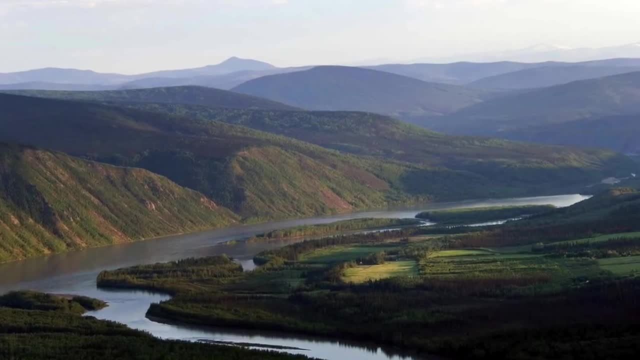 Right, so now let us look at some rivers of these countries, the important ones. First of all, we are looking at the Yukon River, which flows from Alaska, and it is important because of placer gold being found in this river. Placer gold is the tiny particles of gold that are found in the river, which are collected. 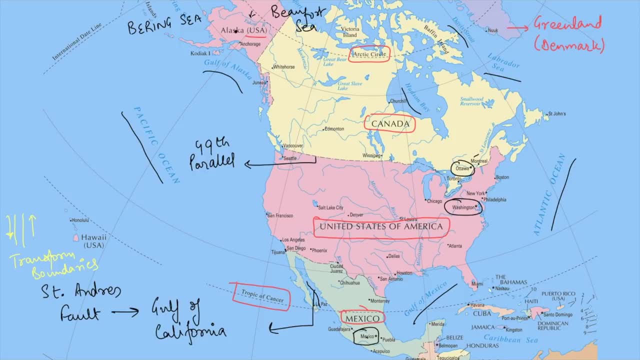 and strained to make gold, and this river is famous for this. Now, which rivers are there in India? which rivers are there in Canada? which rivers are found in Canada? If you want to know which rivers contain placer gold, you have to write it down in. 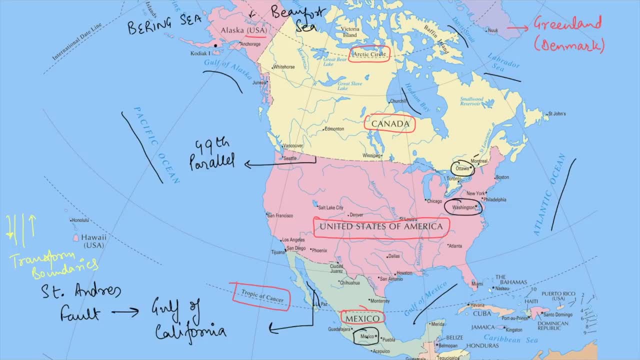 the comment section, I will give you a hint that one river drains into the Bay of Bengal and passes through Odisha Right. so after that you have to look at the Mackenzie River in Canada. Now Mackenzie River drains into the Beaufort Sea. 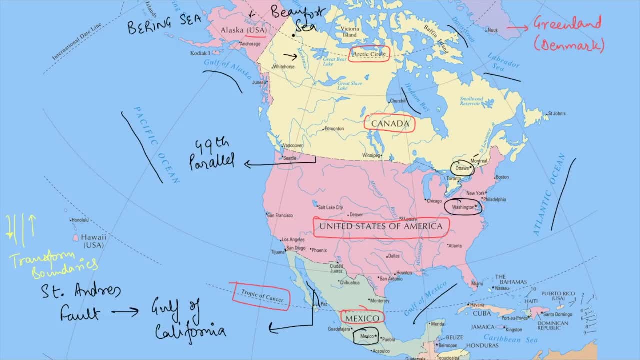 Now, when it comes to rivers, you must remember the location of a river, in which direction it is flowing and in which water body it is draining. This is really important so that if you have an overall picture in mind, it would be easier. 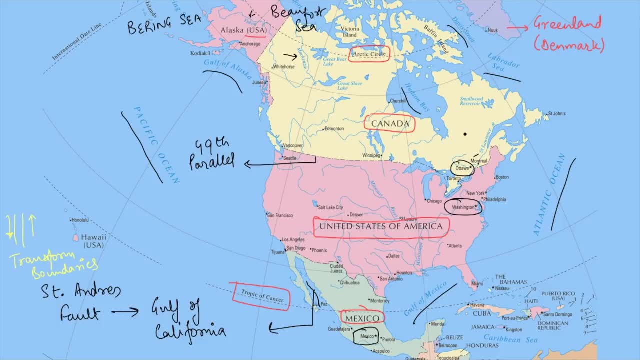 for you to recall. The second river you have to notice here is the St Lawrence River. Now, the St Lawrence River is very special. it is really important because there are so many places here near these lakes where iron is found and that iron was transported through. 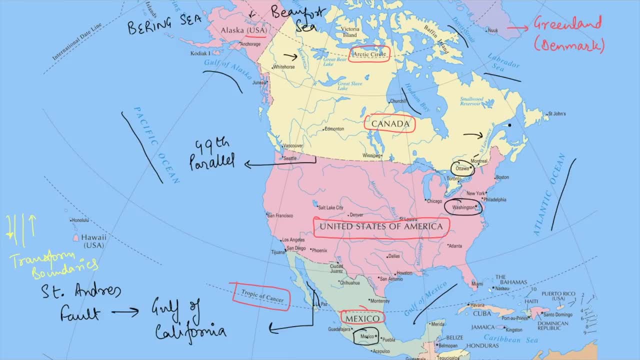 the St Lawrence River since so many years and it is exported from here to Europe. Now, in this area, you have to remember this island as well. This is Newfoundland Island. This is really important because this is one of the best fishing grounds in the world. 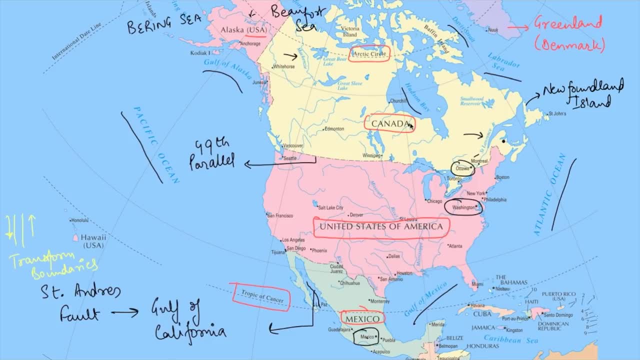 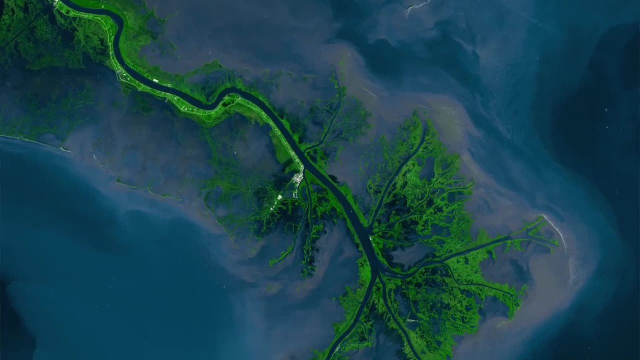 This is one of the best fishing grounds in the world. This is one of the best fishing grounds in the world. Now, if we look at the rivers of the USA, you can notice here Missouri, then Mississippi. The specialty of Mississippi is that the delta here, this is a bird foot delta. 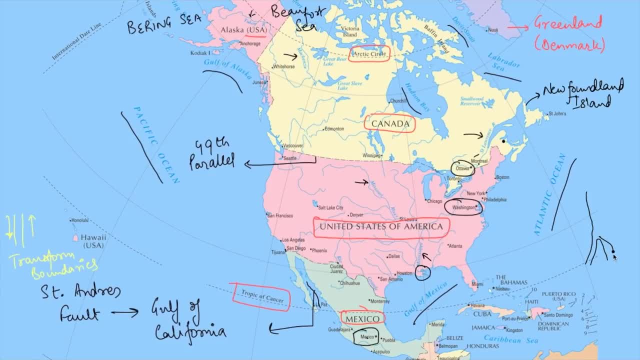 So this is an example of a bird foot delta. If a delta forms such a formation which resembles the foot of a bird, then we call that a bird foot delta. Now, here you can see the Colorado River. The specialty of the Colorado River is that you get the Grand Canyon here in the USA. 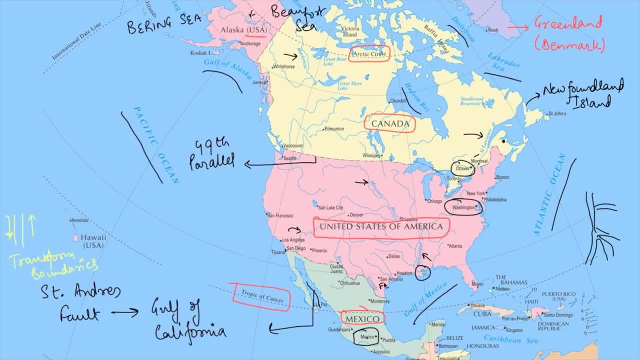 And then notice this river, which is known as the Grand Canyon. This is the Grande River. This is important because this forms a natural boundary between the USA and Mexico, And this river changes its course throughout the year. This is why border disputes keep happening in the USA and Mexico. 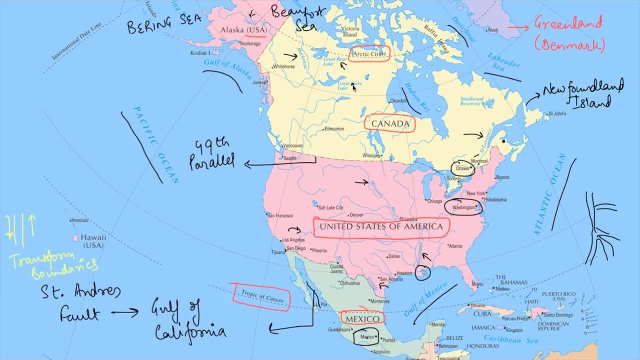 Right now. let's look at some lakes. First of all, we have to look at the Great Bear Lake in Canada. Then we have the Great Slave Lake. Now this is Lake Reindeer And this is Lake Winnipeg. So these lakes are entirely in Canada. 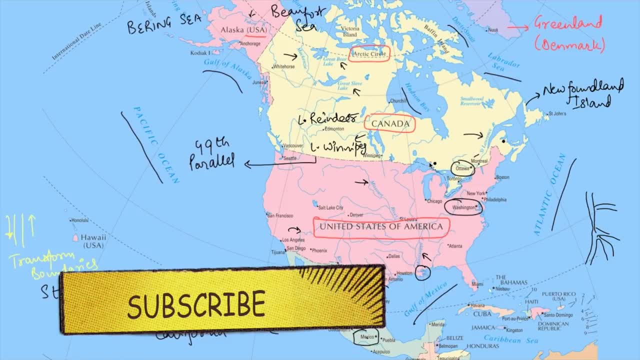 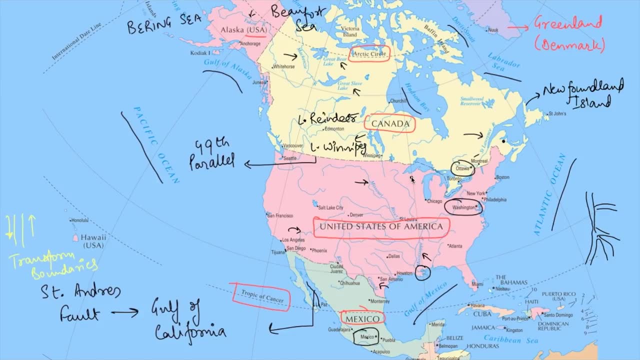 There are some lakes, As you can see 5 lakes here. These are really important, very, very important, and 4 of them are shared by Canada and USA. So to remember them, we will write their short form: S-M-H-E-O. 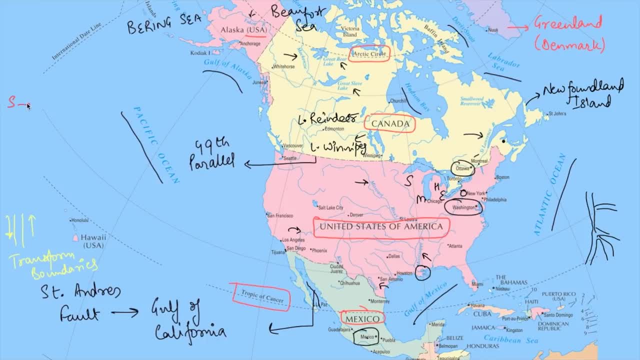 So S-M-H-E-O. Now let's see their full form once. S stands for Superior- Lake Superior, This is the largest freshwater lake in the world. M stands for Michigan, Lake Michigan, H stands for Huron, E for Erie and O for Ontario. Now this sequence is from West to East: S-M-H-E-O. 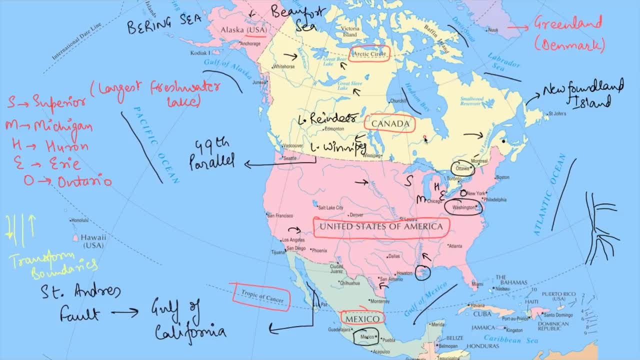 Now, 4 of these lakes, except Lake Michigan, are shared by Canada and USA. Only Lake Michigan, out of these 5 lakes, is entirely in the USA. You have to remember this. Now, when we are talking about USA, let me tell you one more thing: that USA has 50 states, out of which 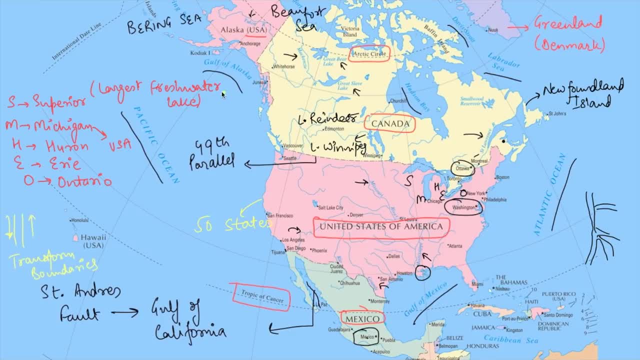 a lot of states are shared by Canada and USA, So this is the sequence from West to East. Alaska is the biggest state And here freshwater means sweet, sweet water lake. Likewise, the largest salt water lake is Caspian Sea and the largest artificial lake is Lake Volga in. 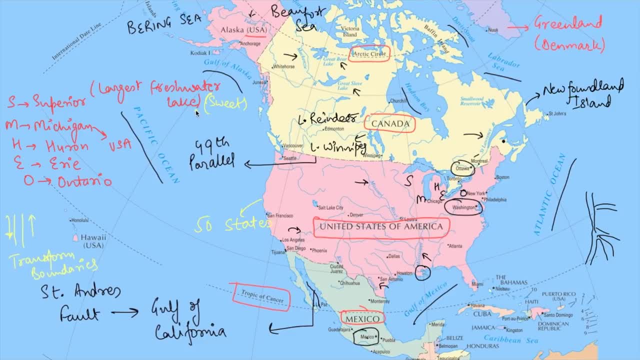 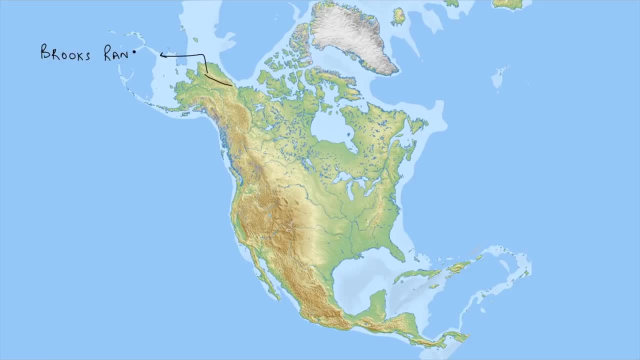 Ghana. Right, so now let us look at the physical map of North America. Now, this is the Brooks Range in Alaska, And this you can see is the Yukon River. Now this is a very big range known as the Rocky Mountains shared by Canada and USA. Now this is the Rocky Mountains shared. 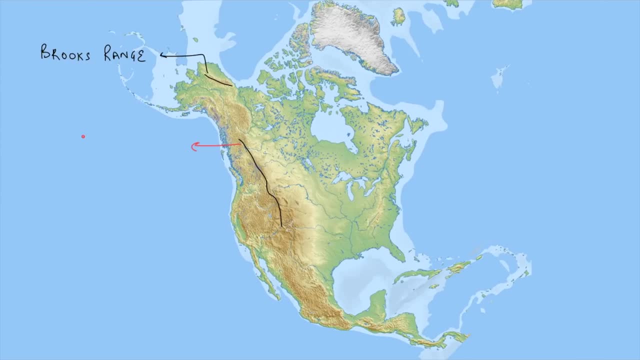 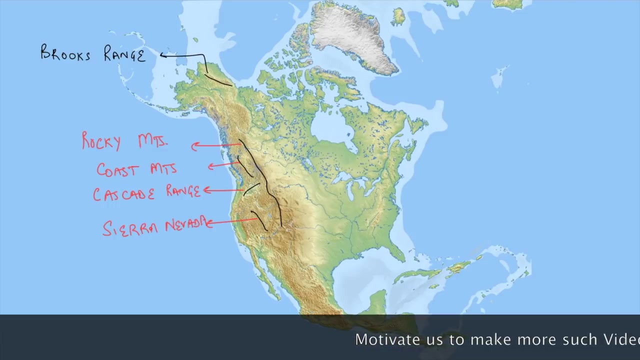 by Canada and USA, And these are the Youngfold Mountains. These are the Coast Mountains. Then we have the Cascade Range, Sierra Nevada. Now, don't get confused with Sierra Nevada. There are two ranges by the same name. One is in the USA and one is in Spain. USA and 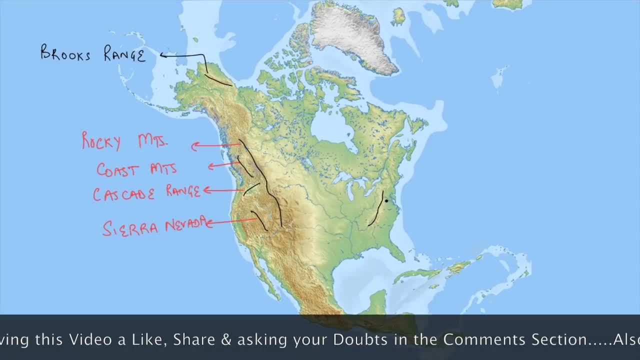 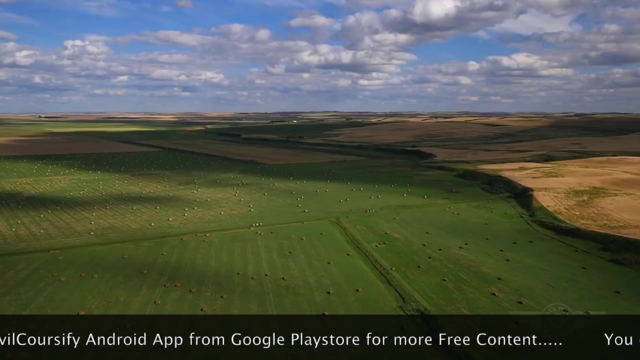 South Africa, USA's Eastern side, these are the Appalachian Mountains. Now, Appalachian Mountains are old, residual Mountains, just like the Aravali Hills in India, And in between these mountains you can find the Great Plains of North America. Now, these Great Plains are: 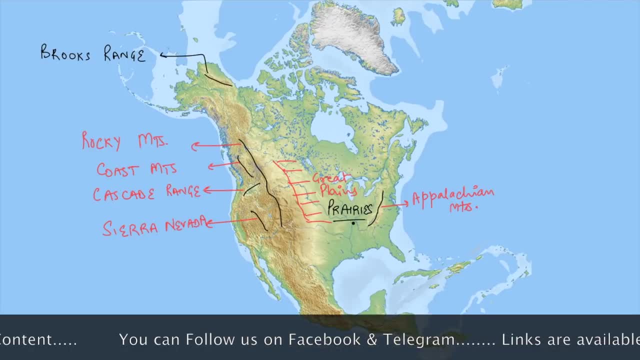 also known as Prairies in North America. These are Temperate Grasslands of North America. Now, Temperate Grasslands, or Tropical Grasslands, are also known as Prairies in North America, also known by different names in different continents. We'll look at them in their respective. 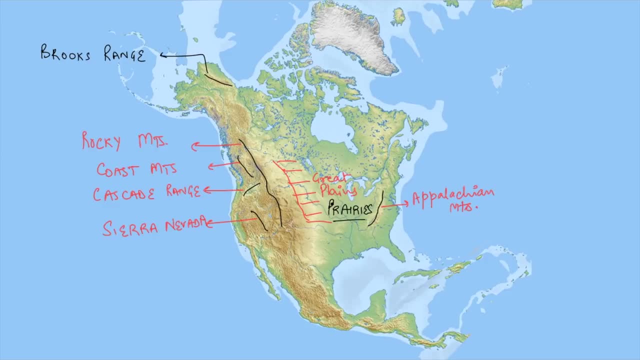 videos. What are pampas, steeps, savannah, etc. In Mexico, you'll have to notice two mountain ranges: One is the western Sierra Madre and the other one is the eastern Sierra Madre. Now this is the isthmus of Tehuantepec, Whereas this is the gulf of Tehuantepec Now in Canada. 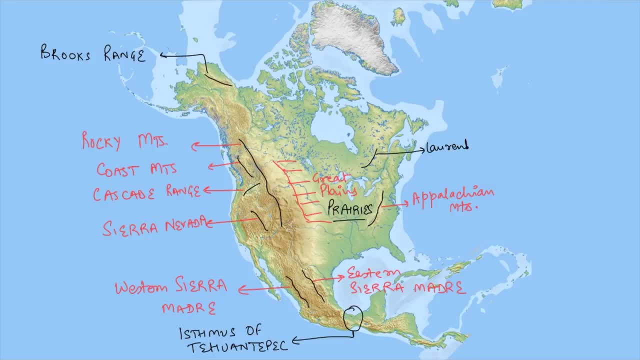 this is the Laurentian Plateau. By the way, Canada has the largest coastline in the world. you must remember this. And the most important part is that you find the Canadian Shield here Abhi. Canadian Shield kya hai? Basically, shield, kya hota hai? 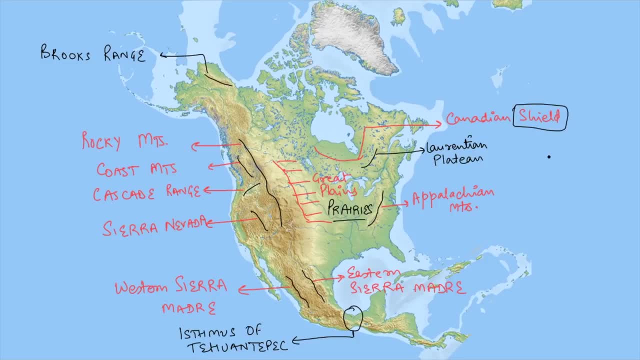 Now a shield is a remnant of Pangea. Pangea ke time se kuch minerals, jo ki abhi bhi continents me milte hain, unko shield bolte hain. So these are remnants of Pangea, the supercontinent. 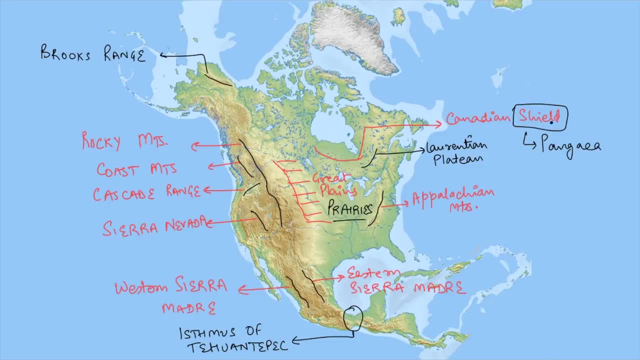 Ab alag, alag continents me shields milti hain, wo ham respective videos me dekhenge. Lekin ek baat hume pata honi chahiye: ki shield me koonse, koonse minerals milte hain, Sabse. 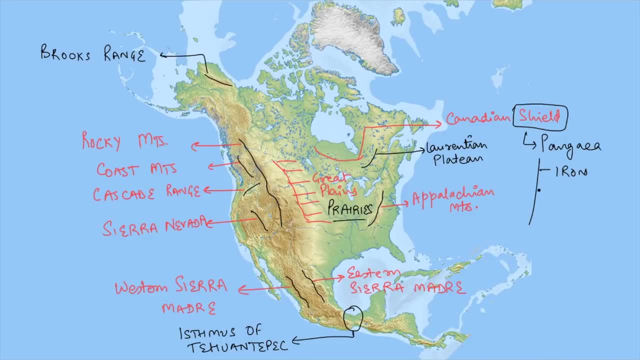 pehle hume milta hai iron, Then uranium, Gold, Copper, Ab copper, ke saath lead, zinc aur silver mi milta hai. Then we get platinum And diamond. Yeh koi fixed sequence nahi hai, Yeh sabhi minerals. 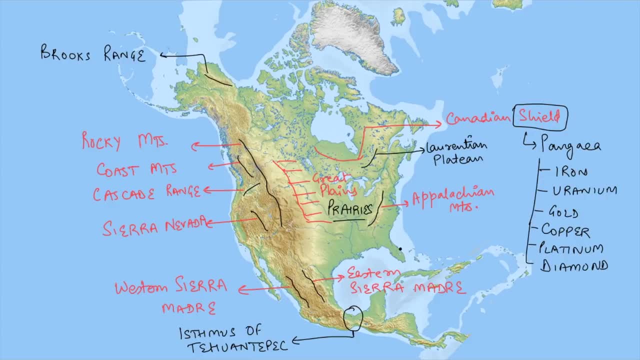 hume shield ke andar milte hain To yeh yaad rakhna hai. Right, so last, this is the Florida Peninsula. Right, so we have mapped the most important features of North America. These are things that you cannot afford to forget. 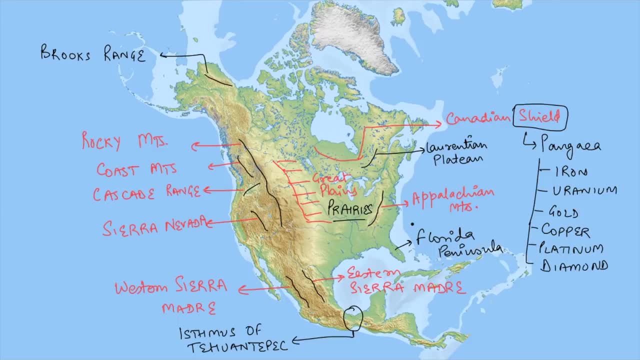 I hope sabko achche samajh mein aaya hoga. Agar nahi saamajh mein aaya hai, so please write it down in the comments section and we will solve your doubts for you. Meanwhile, iss video ko like, comment or share karo and subscribe to our channel, so you never miss a video.